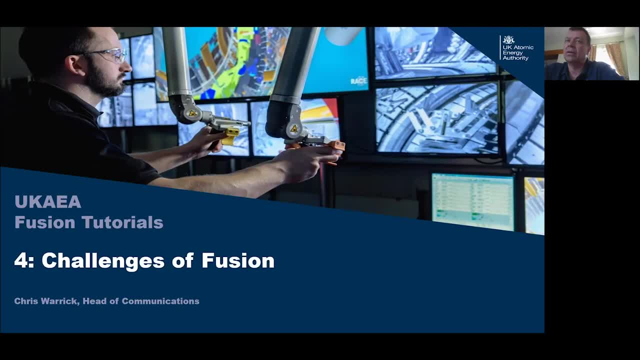 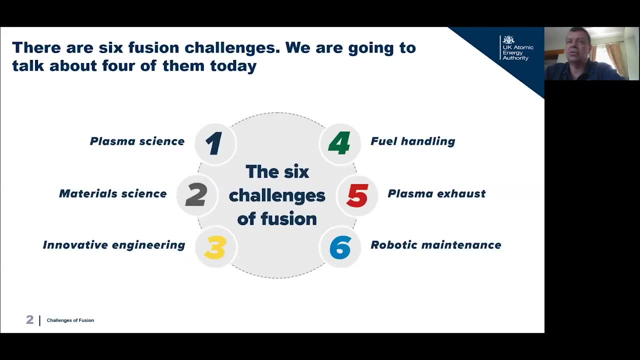 you have got something out of them and understand a bit more about the fascinating world of fusion. So this talk is about the challenges that stand between us and putting a fusion power station on the grid. There are six main challenges. Many of you at the authority will 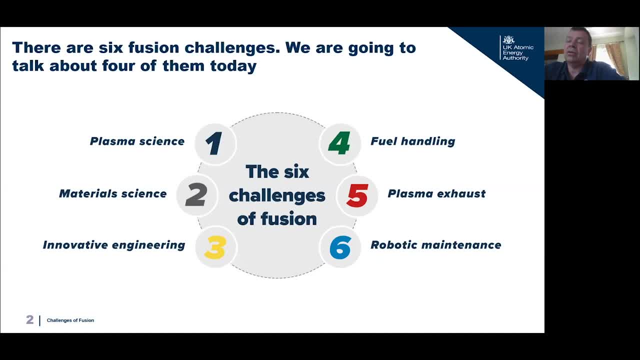 have seen this figure before, As we actually do a work into a lot of these particular challenges. The first is in creating the fusion reaction at all. We need extreme conditions in our plasma, our very hot gas of fuels. to do that We need to heat up to 150 million degrees Critically, we need to 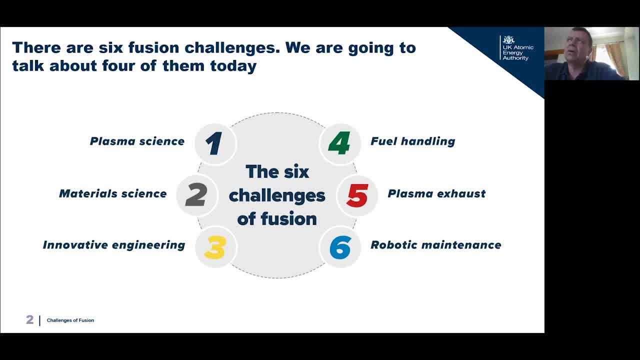 get a plasma to burn, That does not mean to say it is on fire at all. Burning means that it is largely self-heating. It is sustained enough that the energy produced from fusion, in particular in the helium, keeps the plasma hot enough. 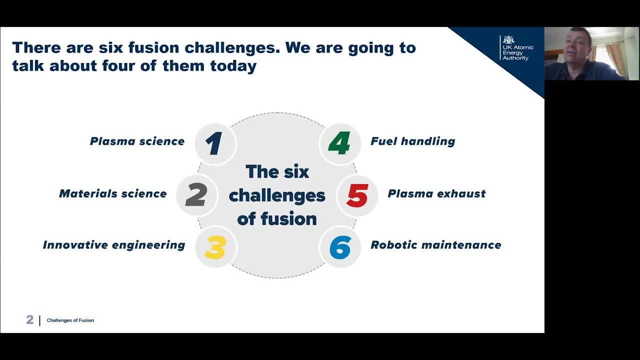 And sustains it. We need to sustain the magnetic field to hold that in place, And we will talk a little bit about that in this talk. We will also talk about the challenges from materials, which is truly huge and very diverse. We need materials that can cope with high heat loads. 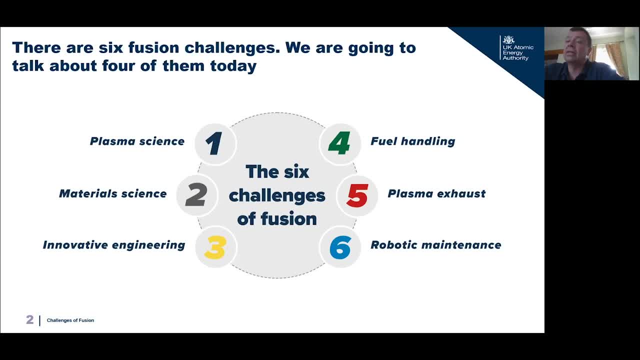 materials that are resistant to holding tritium, materials that are resistant to the damage and the radiation caused by neutrons, And we will touch a little bit on that. Innovative engineering will come in a future talk about how to put a fusion power station together. 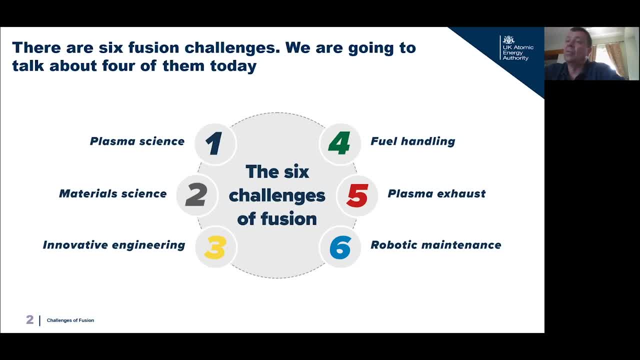 will come in talk number five, as will fuel handling. we need to look at breeding and using the tritium fuel in particular, which is much more difficult to handle than the deuterium that we use. i will also touch in this talk on on how we exhaust our excess heat from the plasma. 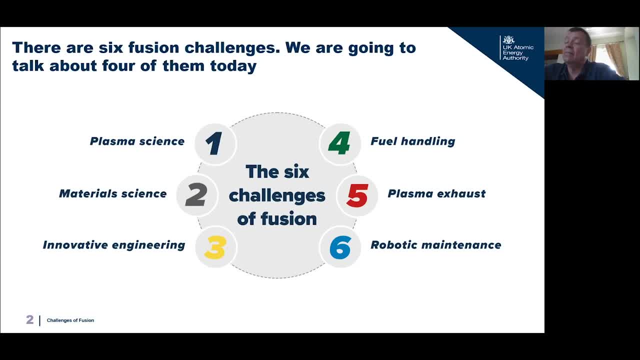 we produce too much heat in there. we need to get rid of the excess and we need to get rid of the helium once it's cold. and i'll also talk a little bit about robotic maintenance and the huge challenges that we face there. these are some of the really practical technology and engineering. 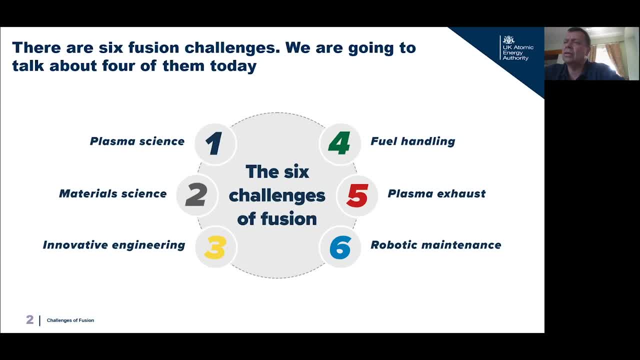 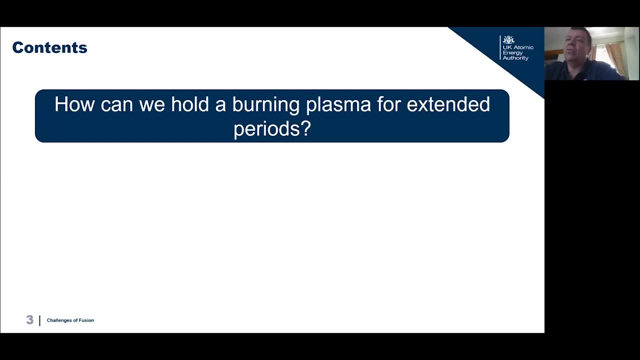 issues that stand between us and putting a fusion power station on the grid, and i will- i will touch on on each of these in turn, so to to emphasize: how can we hold a burning plasma for extended periods? again, a burning plasma is a plasma that is sustained, sustained and heated by the action. 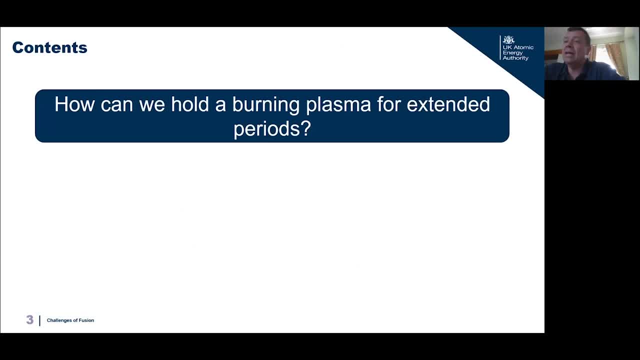 of the plasma itself. largely that is from the helium that we produce and can sustain, keep that plasma at fusion type conditions. but we need to work out how we can produce long-lived magnetic fields for that to happen. so we'll talk a little bit about that. what we do with that heat. 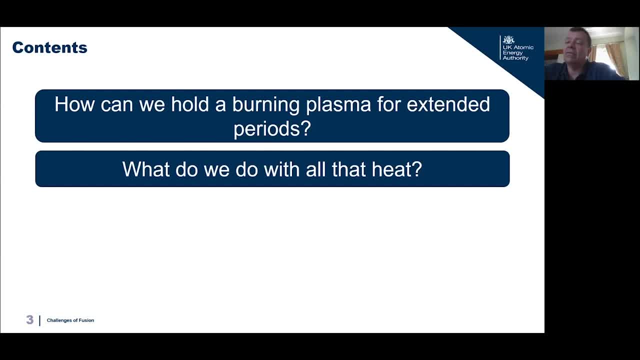 the excess heat that we no longer need. how do we get rid of that? that requires the plasma to touch material surfaces. how can we deal with that? what generally do we want our materials to do to survive in this environment? and i i'm? there are various issues around that, so we'll touch on on those very 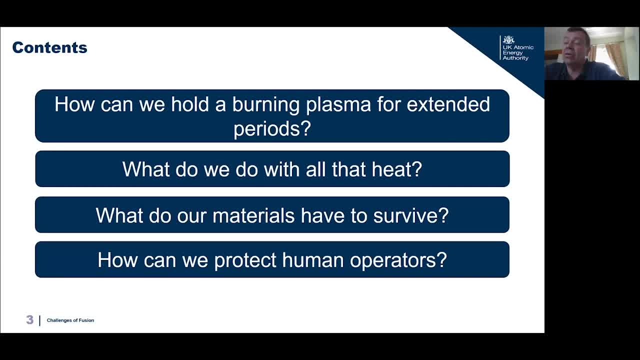 very briefly: um and how can we protect humans? we cannot send humans going into the machine. um, this is a radioactive process and the interior of the fusion device is radioactive- mildly in the case of jet, but more so in the case of a future power station. we need to. 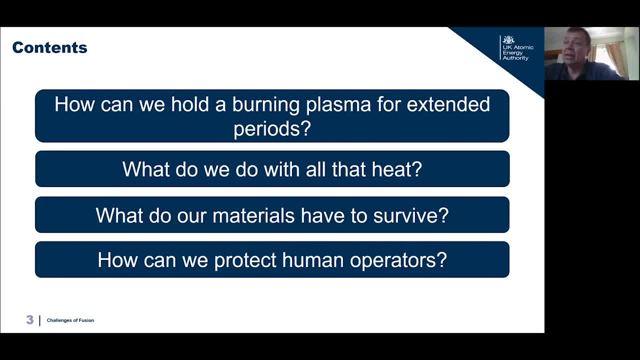 devise remote handling techniques that work both inside and immediately on the outside of those those devices, um so that we are not caught out with a problem that we can't fix robotically. um, so we'll. we'll have a quick look at all of those in just a few slides on each. 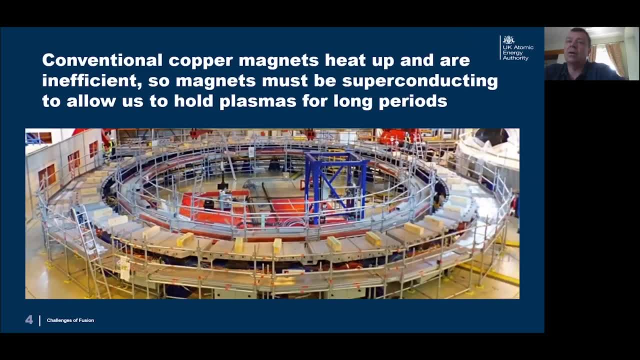 the first on on a burning plasma. we require, um, our, um, uh plasmas, um in the. in the case of a burning plasma, we require them to to last for potentially continuously, but certainly many hours at a time. and if we contrast it with that, with what jet can do with the minute jet can only operate for. 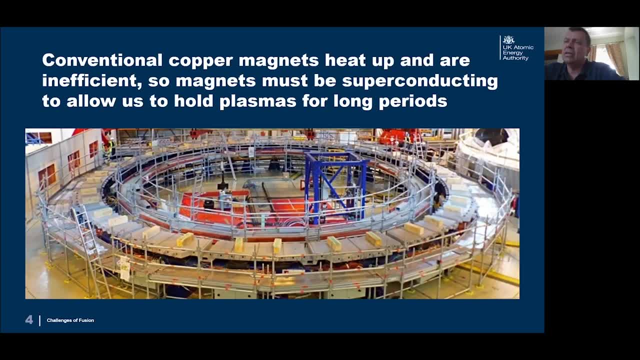 30 to 40 seconds, maybe a minute at most. one of the reasons- and there are a few- is that jet has conventional, as we call them, copper magnets. copper coils- uh, heat up. in a previous tutorial we talked about the action of the electrons flowing through a material. 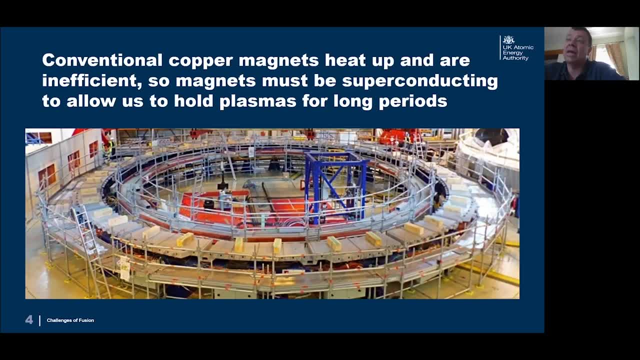 and the fact that they will collide with the atoms and heat that material up, and that is wasted energy. um, so, because our copper coils on jet heat up, if we run for really long pulses, our coils start to get too hot and won't run any longer. so, um, there is a material, there are a. 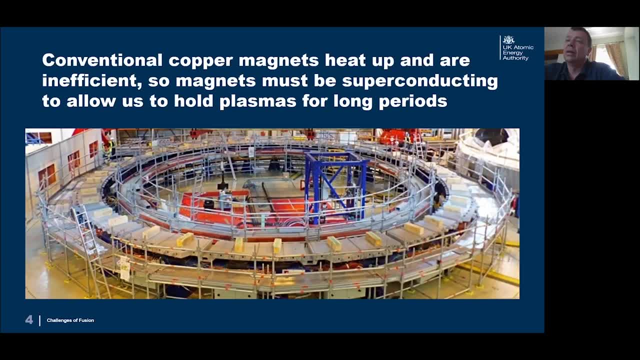 suite of materials, and particular ceramics in particular, that are so-called superconductors. superconductors are materials that exhibit zero resistance. there is an internal rearrangement of the particles that essentially means the electrons can flow completely freely, not colliding with anything and exhibiting essentially zero resistance. so this is a real game changer. 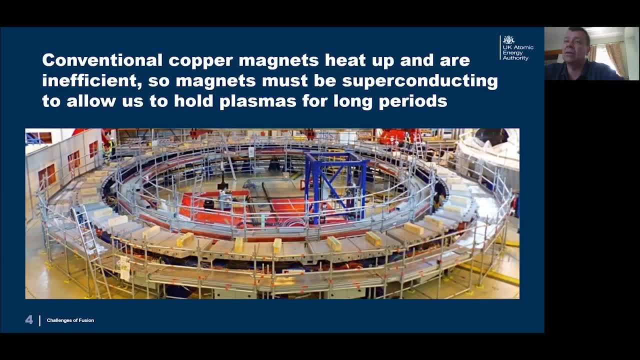 for fusion. if you can make your magnetic coils out of superconducting materials, then you have no resistance. they don't heat up and actually, once you've set the current running around them from your power supply, you can switch off that power supply and the current will continue. 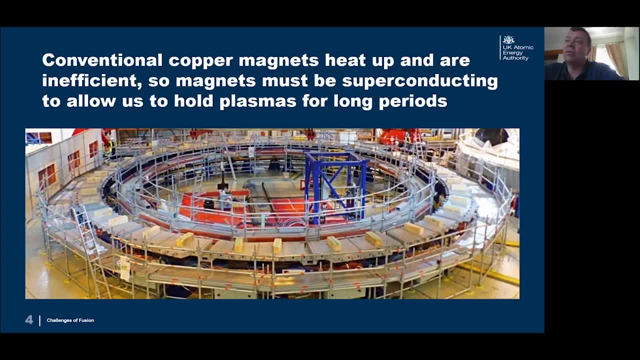 to run um this. this means it's much, much more efficient. you're not constantly driving current around the coils to make the magnetic field. you start that current off and then just let it go and essentially you're getting your magnetic field for free, except the superconductors required. 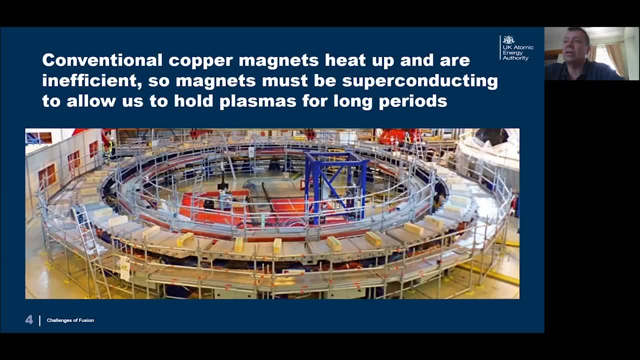 are required to get very cold before they're superconducting, so you do need to think about the energy you use in cryogenically cooling the coils. we'll come to that in a second. but these superconductors we know are going to be very, very important to hold plasmas and hold burning plasmas for long periods of time and make 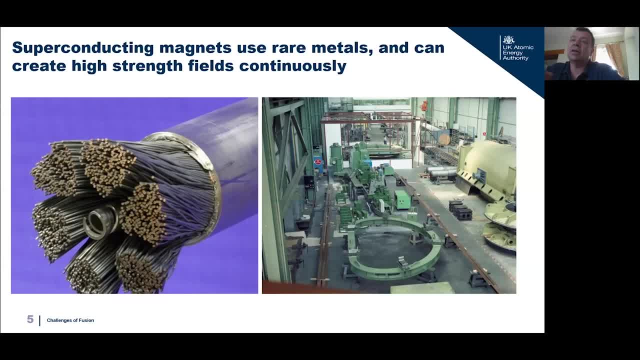 a future power station. economic superconductors are around and have been known about for many, many decades. they typically um, are exhibited in in quite rare metals and ceramics and alloys. they can create high fields and they can do that continuously without heating up, as i said, without exhibiting any resistance. and on the left here is some superconducting strand. 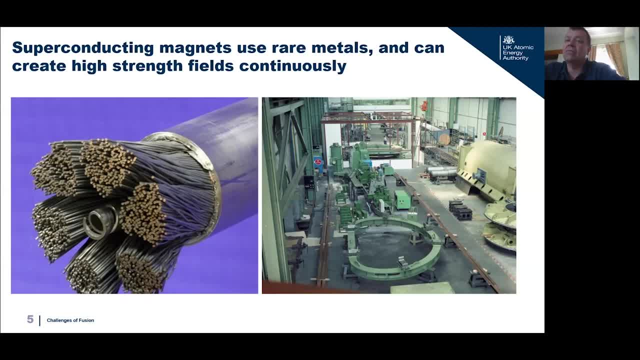 um a picture of some superconducting strand. all of the conduct conductors in there are superconducting if we can get down to the really low temperatures we need. and on the right are some coils um being wound for eater. eater is the next machine along from from jet um will use. 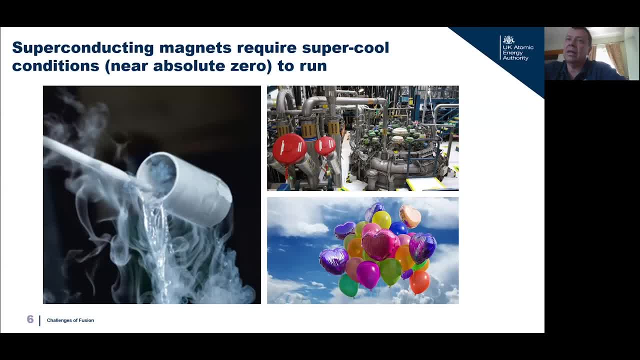 superconducting coils. um, i'll come on to that in a second um they do require very, very cold conditions. this is the the disadvantage. um we actually need for the superconductors we're going to use on eater and and indeed in other fusion experiments. at the minute, running the superconductors, we need the temperatures. 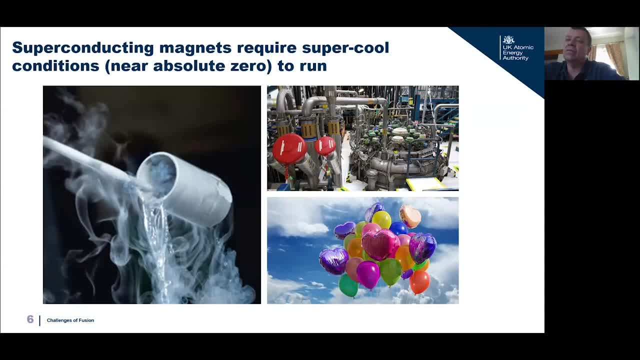 to get down to near absolute zero. um in the case of the superconductors we know about at the minute. um then, that is liquid helium temperatures. liquid helium helium liquefies at just four degrees above absolute zero, that's, minus 269 degrees centigrade um minus 273 degrees. 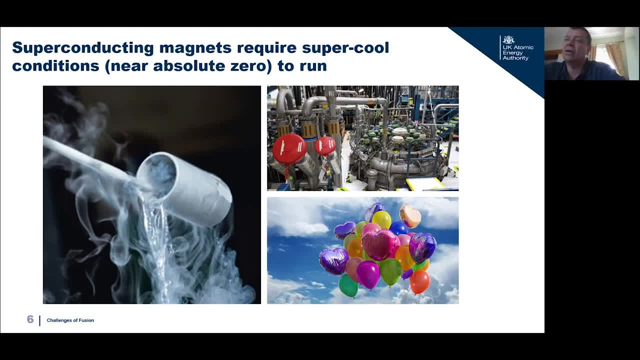 centigrade is the lowest temperature anything can get to, so we're right down at the very bottom. i mean in the mid 20s of 2021. we're in the mid 20s of 2021, so it's a very pretty late period. 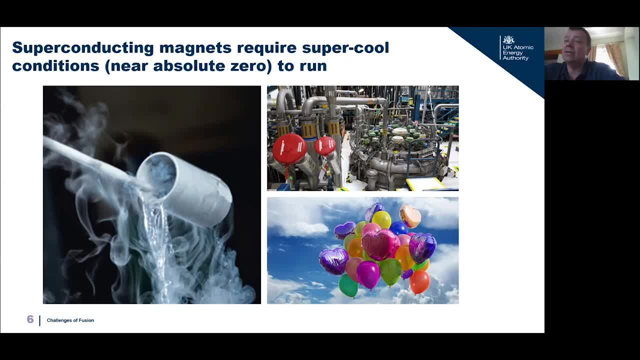 of time, the, the, the, the, the, the, the. these particular materials are superconducting only when we cool them at that kind of temperature- um and liquid helium is, is we. we have to put quite a lot of energy into manufacturing. that at the top right is a picture of a cryo plant we have. 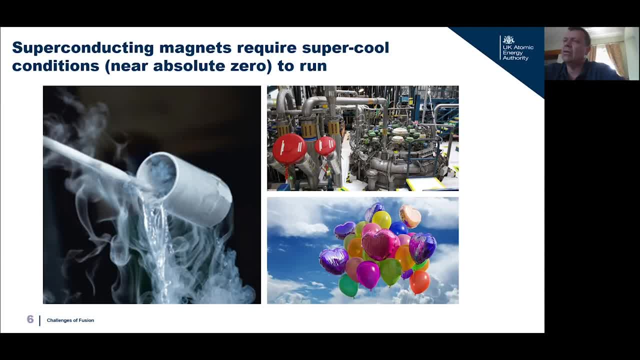 a big cryo plant producing liquid helium um and indeed using liquid nitrogen as well, and we we have deliveries of liquid nitrogen to column out cry plant um and other uses, especially on jet, and indeed we're looking to put a cryo plant and cryo pumps. 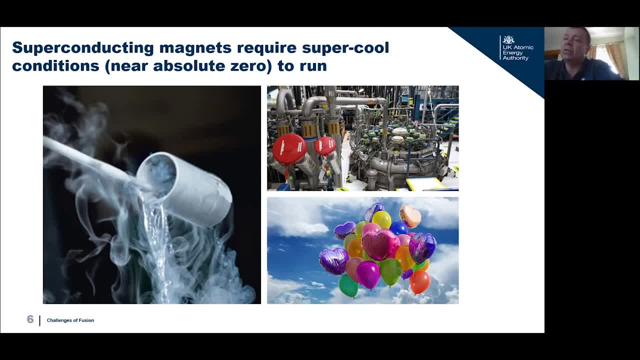 into mast as well as we upgrade the mast machine so we can take that helium and heat it down to these crazy cold temperatures, which requires energy of course, and on the the left you can see, liquid helium has absolutely fascinating physical properties. liquid helium for all sorts of reasons, but once we can cool particular coils down to those kind of liquid helium temperatures, 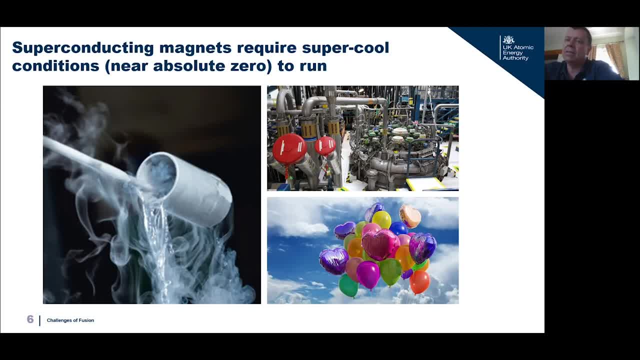 they will be superconducting and this will be a big, big technology that needs to get used in future fusion power stations to make them economic. we need much less energy to drive the cryogenic plant than we we would use if we used conventional coils, so it certainly does. 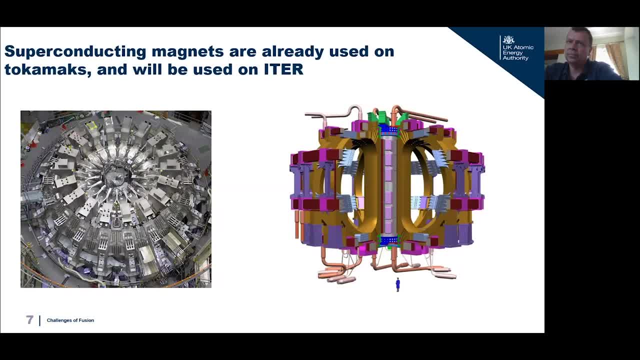 save us an awful lot and start to turn the economics in our favor. we talked about these being vital. on on on ETA. there is a picture on the right of the superconducting coil set on ETA with a with a person. to give you some sense of scale, these are huge. in the case of ETA, these are neobium tin. 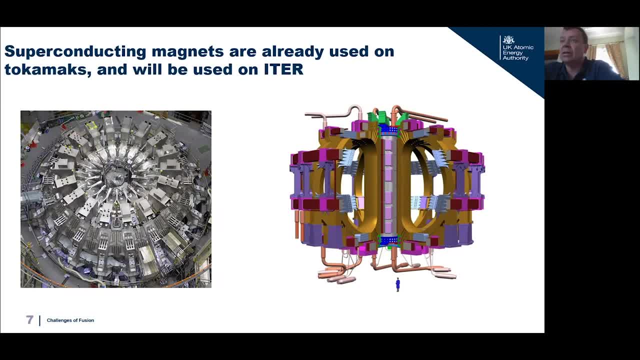 and these are the biggest superconducting magnets that the world has ever made. these are absolutely huge. these are 12 to 14 meters high and indeed some of them have already been wound and tested. so this really is pushing the boundaries of what we can do, but absolutely. 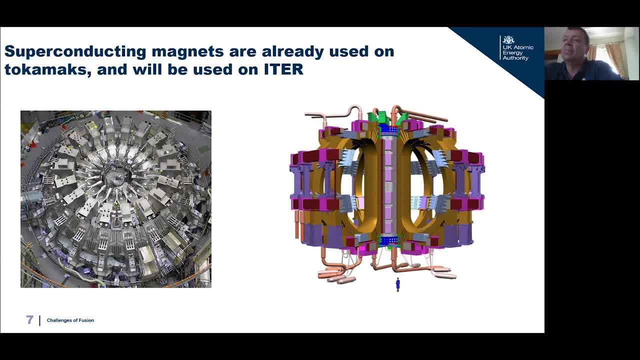 vital, ETA will. ETA will produce 500 megawatts out, but it's a requirement, for magnetic fields is much, much less than on jet. so we actually will produce more power out a meter than we put in and ETA will start to demonstrate some kind of gain towards a fusion power station of the future which will exhibit 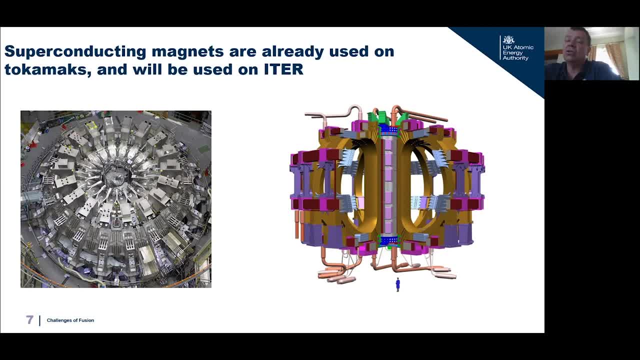 significant gain to make it economic. on the picture on the left is a picture of JT 60, which is a large up recently upgraded tokamak in in Japan, similar to the one we've seen from bastards size and scale to jet. it doesn't have remote handling of deuterium but it does. 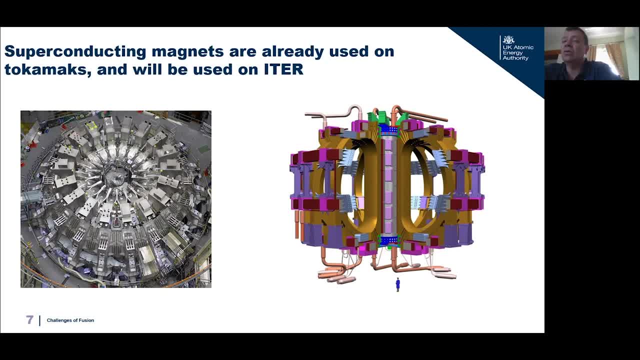 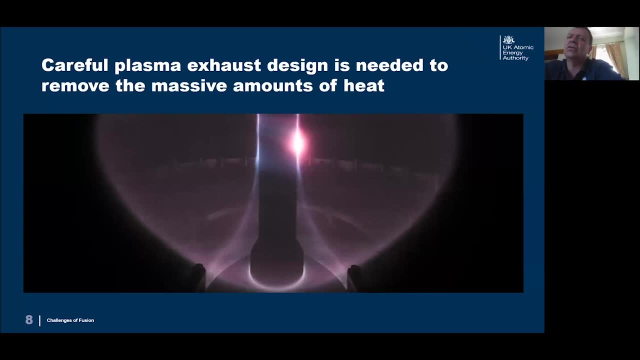 now have superconducting coils, so JT 60 would do a lot of work in preparing the way for operating the coils. I need to. understanding how they work there is very, very important. so that's superconducting coils and they are really important, not just infusion, but in other industries. we're going to look. 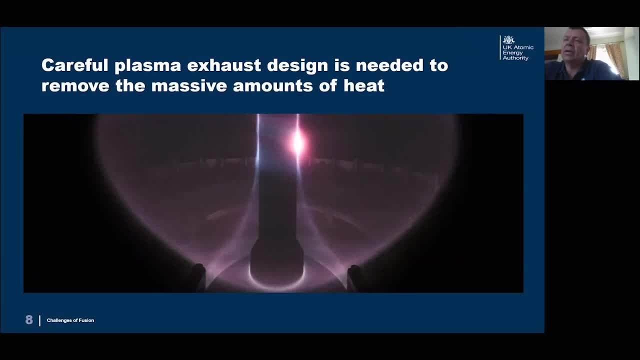 a little bit now at how we get rid of the excess heat we talked about. here is a picture of a plasma on mast. we also, of course, produce very high temperature plasmas in jet. there is the plasma. we are magnetically confining it, getting it. 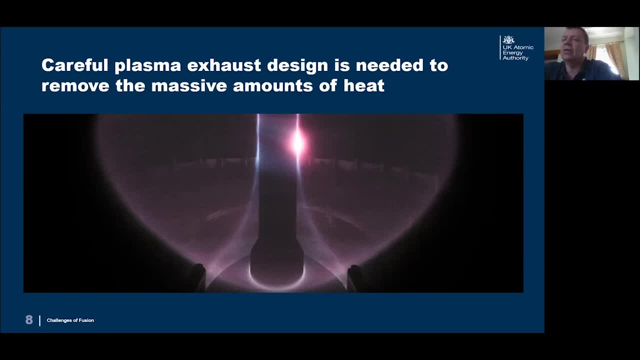 as hot as we can in the interior so that fusion conditions prevail and we start to see fusion. we start to produce neutrons from that fusion reaction, um. but we almost produce too much heat for our own good and we need to excess that. in addition, the helium that we produce is a very high temperature plasma and 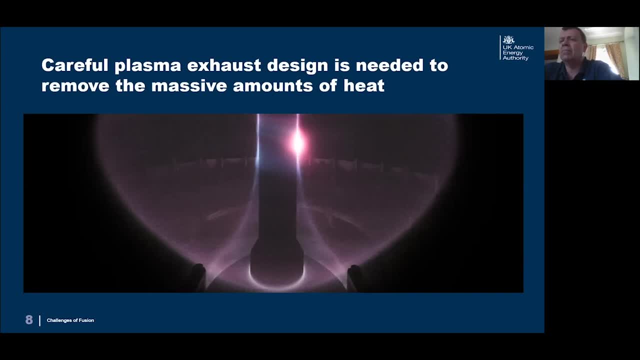 produce in there that stays in the plasma. we talked about that burning plasma. the helium, as it cools and collides with the incoming deuterium and tritium, helps to heat and self heat the plasma and that can be a very powerful mechanism in much larger power plant scale devices. and that's certainly what 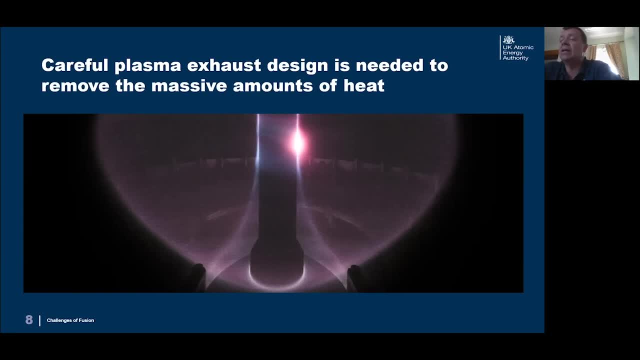 we assume in future devices that it will largely be self heated by the helium. but once it's cold it's a. it's a contaminant, it's an impurity we need to exhaust out. so we need to find a way of getting rid of it. you'll note in the bottom. 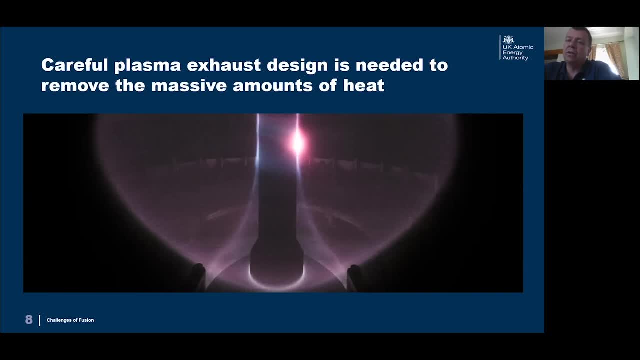 of masked and many of you will see in this pictures before the very bottom that we're focusing on. there is where we deliberately cross the edges of the plasma and to plasma streams, then will penetrate into what we call the diverter region, where we divert the plasma streams and we pump away the excess heat. 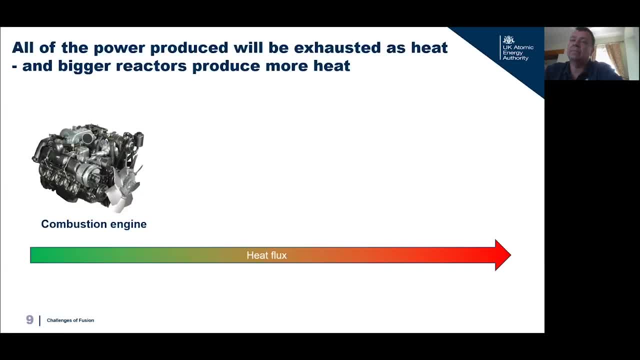 and particles that come out through the edges of a plasma. those diverters have to withstand some kind of heat load. for some decades now we've looked at this problem- and this is a long, long andеш originating shortly after the嘉mert- and realize that it is quite a big issue. 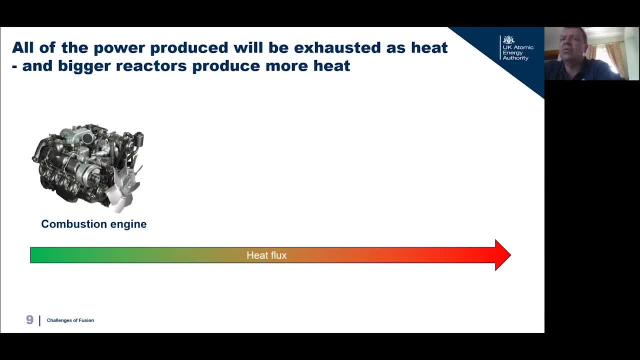 Materials deal with heat loads all the time, but it's how much heat load they deal with. that gives us the kind of headaches we've got with fusion. And then I will talk a little bit about the potential solutions as well. There is a combustion engine. 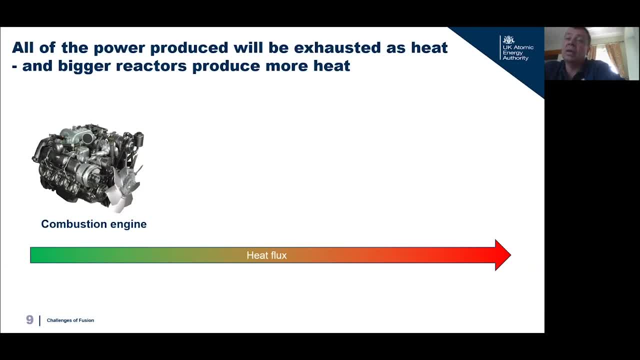 that many of us have in our cars That has to deal with heat loads As the cylinders move round. we actively cool an engine with water and with a combination of water and air, But we do the materials in the engine do get up to heat loads of something. 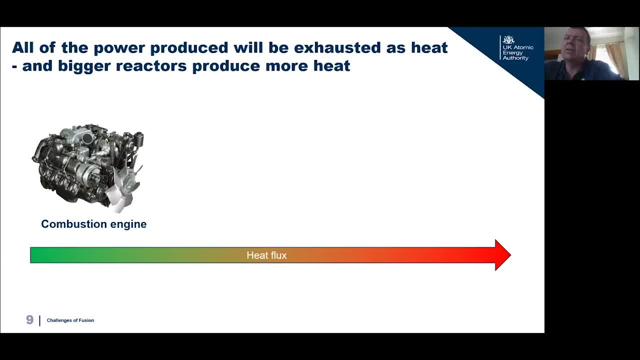 up towards 100 kilowatts per square meter. These are perfectly able for standard, relatively standard, materials to deal with. We're much clever at that now. And indeed a car engine, if well looked after, could last for up to 20 years. 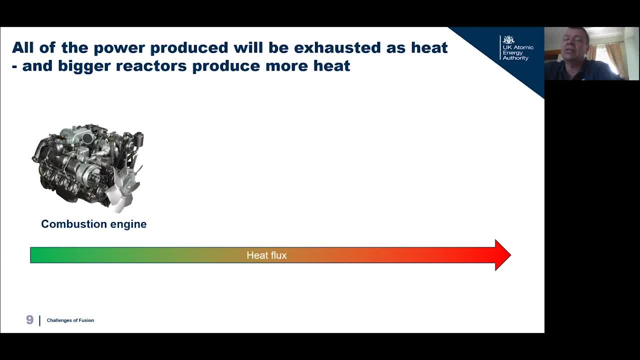 many hundreds of thousands of miles potentially. So that's the kind of technology we know about and we can deal with. If you go up again in scale, you're getting to something that's much more difficult to deal with. So a spaceship reentering the Earth's atmosphere. 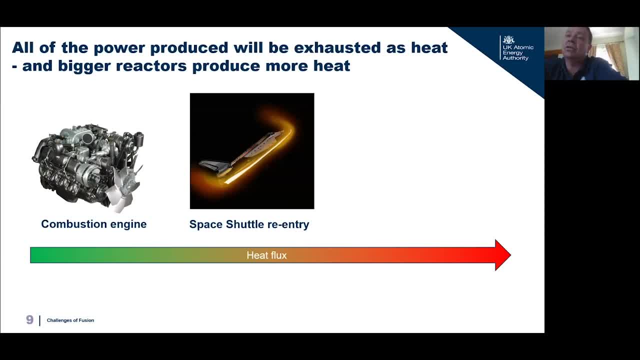 this is a picture of the space shuttle, but you could equally look at the Soyuz capsule bringing astronauts back from the ISS. has to withstand just for 20 minutes or so. pretty extreme heat loads up to a megawatt or two or maybe up to five megawatts per square meter. 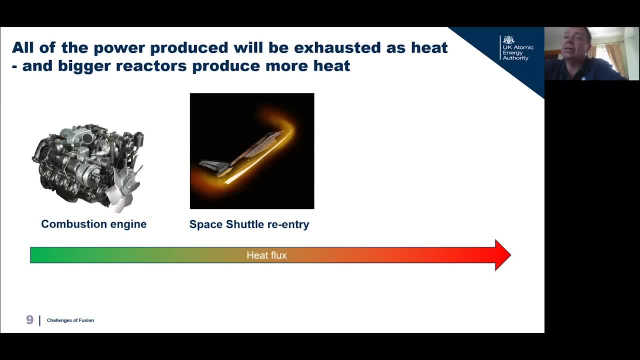 Really difficult to do that, even for that 20 minutes, And that requires clever ceramics and clever design to make sure that that happens properly. And that is the kind of power levels we exhibit on a fusion diverter. We'll talk about that again in a second. 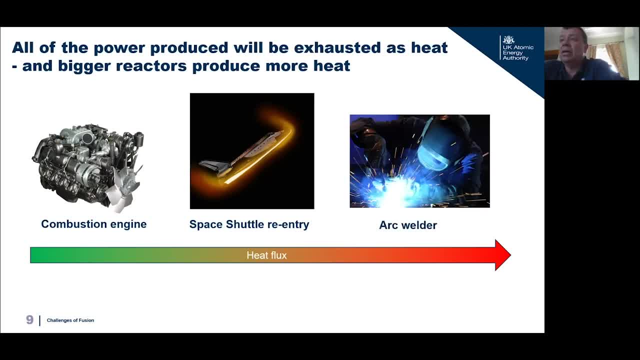 And beyond that, we're up to where we deliberately deform and change materials around An arc welder deliberately melts and reforms joints And that is not where we want to get to. But with fusion, we're currently in the middle and in a region where we have to be very, very careful. 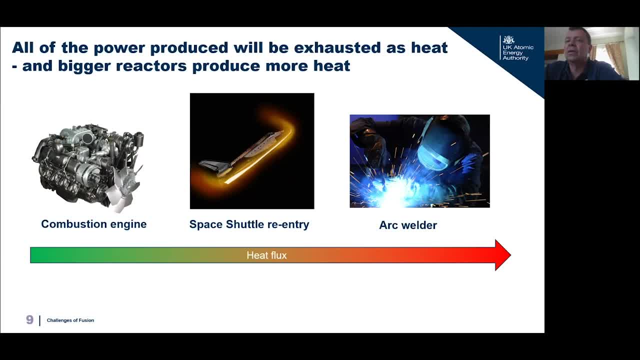 about the materials we choose and how often we'll have to replace them. So that's the kind of race that we're in: The range of heat fluxes materials typically have to deal with in particular scenarios today. So here is a still image of a plasma in JET. 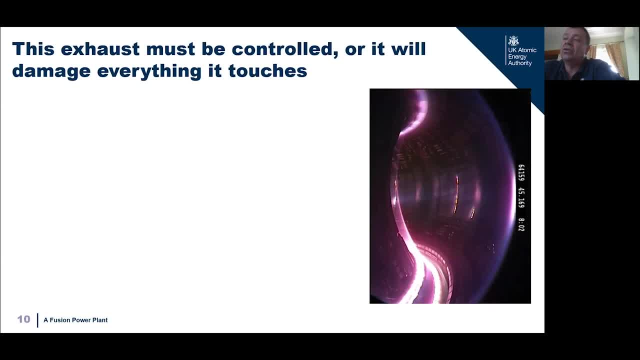 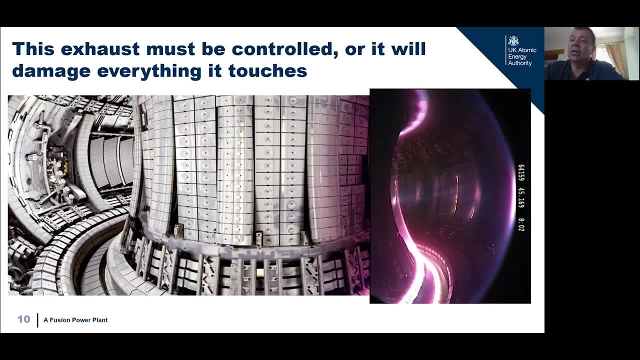 JET has a diverter at the bottom. You can clearly see the two streams of plasma striking at the very bottom into two grooves of the diverter region, And if you look at an empty picture of the vessel, those grooves become much, much more obvious. 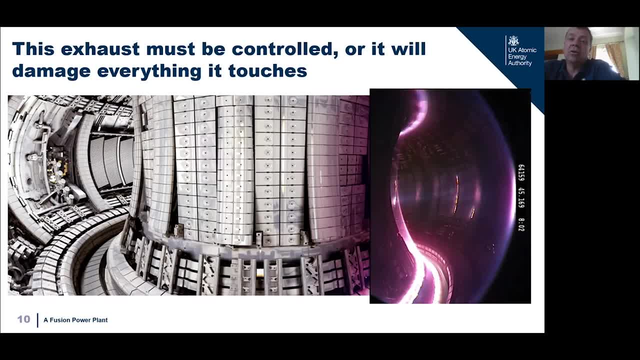 on the left. there You can see at the bottom where we've got. you know, you've got angled plates in the middle and two troughs, essentially that run all the way around the machine. We magnetically steer and cross the two edges of the plasma. 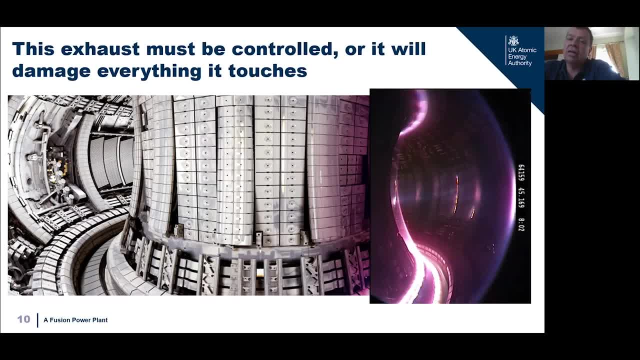 and our two plasma streams move into that region and strike those plates, those special plates at the very bottom of JET. Those plates are made of tungsten, one of the hardest wearing materials we know about, And we know that in a fusion in a JET plasma, 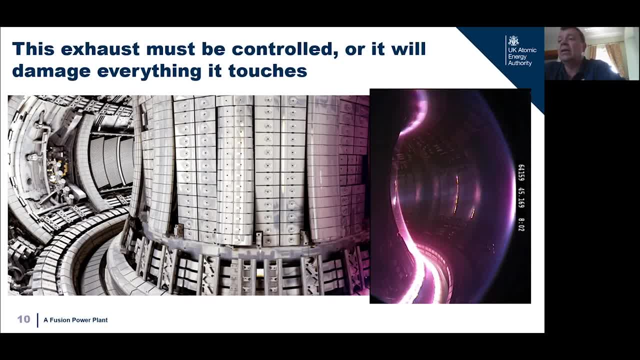 and indeed in a future fusion, in a future power station, the helium that we make, as well as the deuterium and tritium, will make its way to the edge of the plasma, be swept down to this region and pumped away. 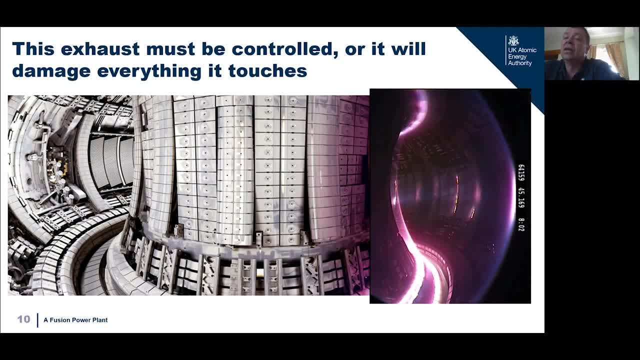 Underneath there on JET is a cryopump, a very cold surface that essentially condenses and sucks anything away that touches it. The kind of power loadings we know about and that can predict for future power stations are of the order of spaceship reentrant power levels. 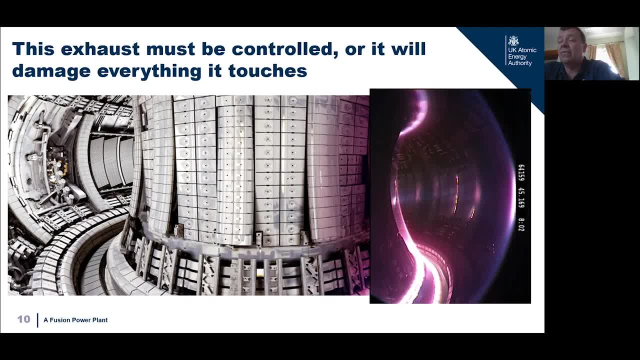 a few megawatts per square meter. But in the case of for us we would have to withstand that in JET just for a few tens of seconds, but in ITER an hour or two in a power station of the future. 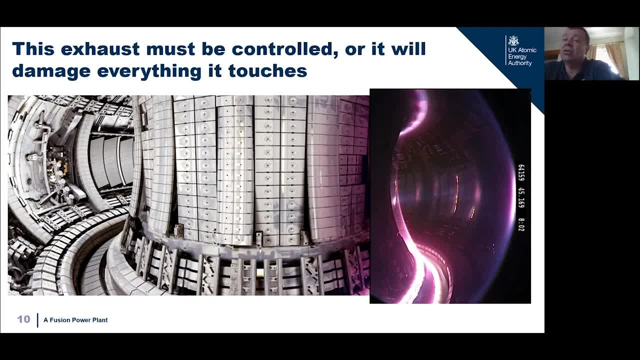 days and days and weeks and weeks, years and years, potentially up to 40 years, and no material will cope with that. Tungsten will do a pretty good job, but within a few years we predict that we'll need to change the tungsten around. 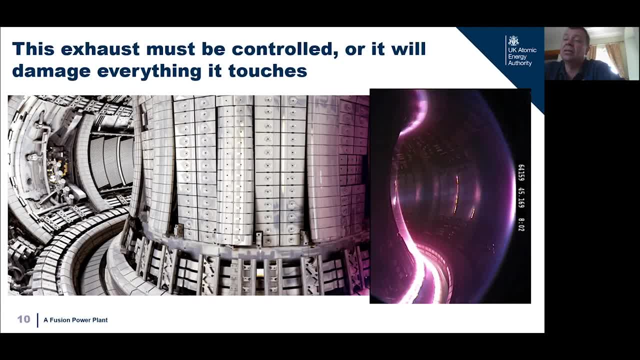 That requires getting remote handling in changing the tiles and this is all affecting the economics. We know there's an issue coming- Tungsten can help us- but we know that we need to try and do better, And what we're gonna do on the upgrade to MAST. 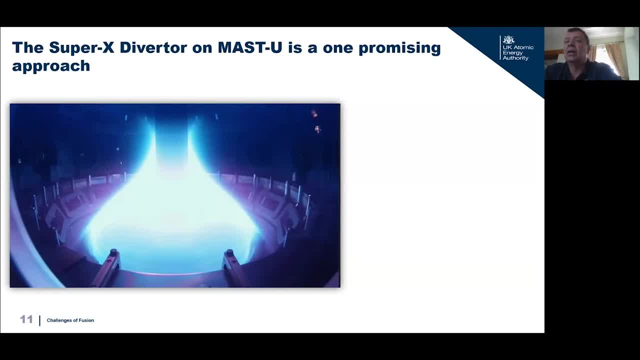 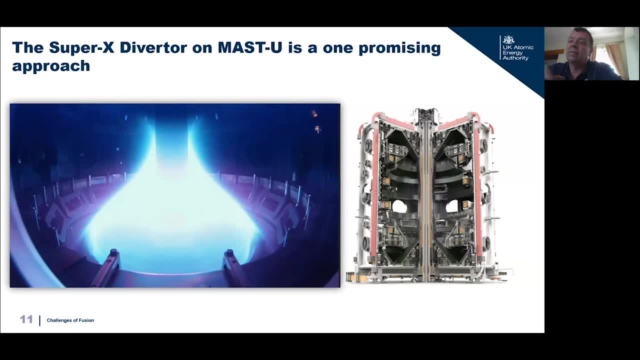 is something called the SuperX Diverter. You may well have heard of this. This is a clever diverter configuration and there is a picture of the diverter region in MAST. Here is the upgrade to MAST, currently finishing off final commissioning. 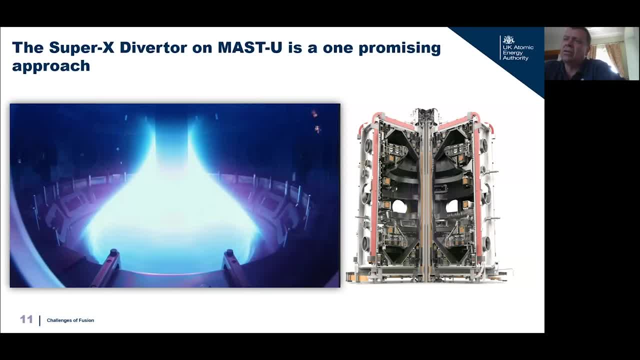 and hoping to start running later this year. And MAST has a diverter top and bottom so that helps you straight away And spreading and sharing the load more evenly. We deliberately magnetically steer the plasma streams much, much further into those private regions. 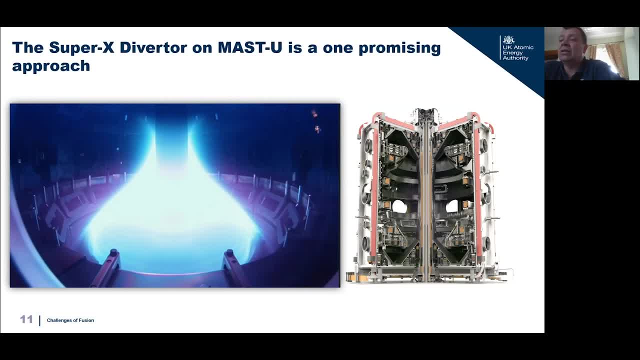 at the top and bottom. That acts to do two things. First of all, by doing that we deliberately spread out the power, loading much more across the plates. The plates are much bigger here than they are in jet And by traveling further it actively cools itself. 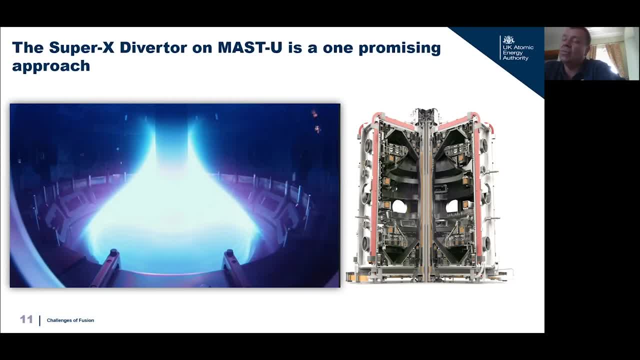 so that by the time we impact on those plates, we expect- and we don't know this for sure until we run the experiments, but we expect- to be up to an order of magnitude 10, down from what we exhibit inside jet. That gets us down to the kind of power levels. 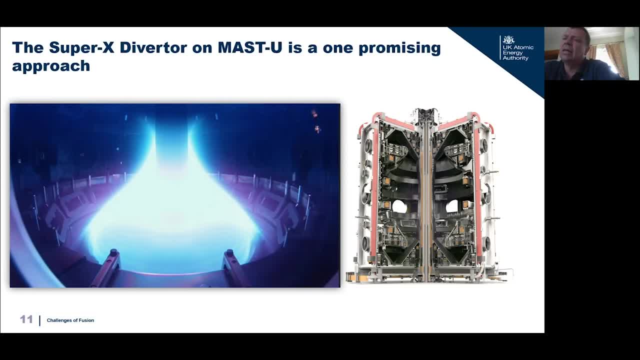 found in a car engine, stuff that we're much more used to dealing with. If that works- and there is a big if, because research science is like this, but if that works, that's a real game changer. for fusion. Here is a diverter design. 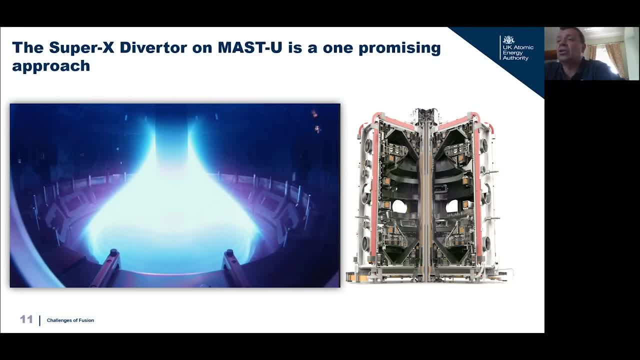 where the power loading is much less. You don't have to get in as often to change the tiles around. That improves the economics and the efficiency and the viability of a future power station. So this is a really big deal and one of the biggest things. 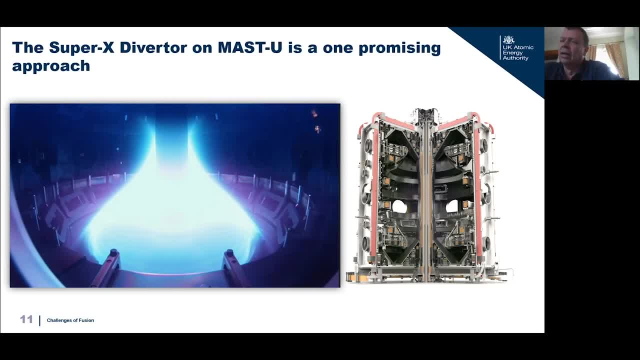 if not the biggest thing that MAST will look at. ITER won't have a super ex-diverter, but indeed power plant designs beyond could easily do that, depending on the results we get from MAST upgrade. So you can see that exhausting the heat is a big issue. 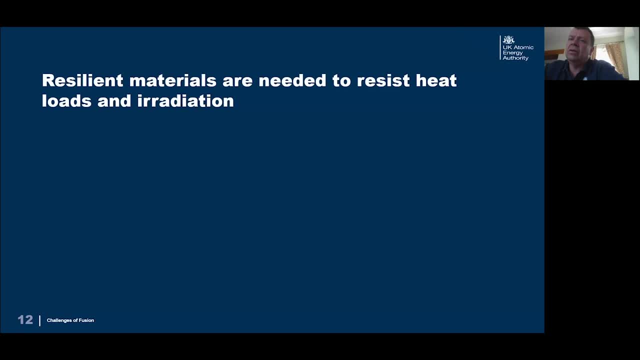 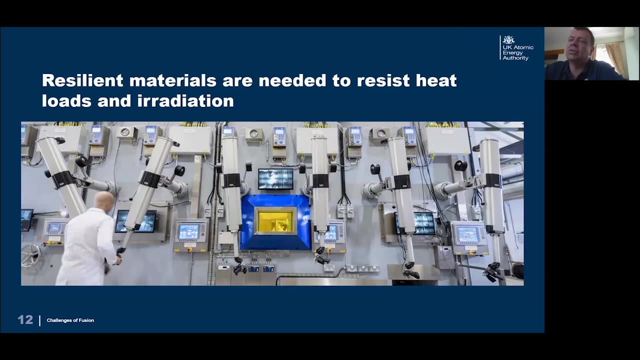 That's where we certainly need heat resistant material. We also need materials to do many other things and exhibit certain properties to minimize the damage caused by the very harsh environment of a fusion power station. Our materials research facility is looking into all sorts of materials and just starting to do that work. 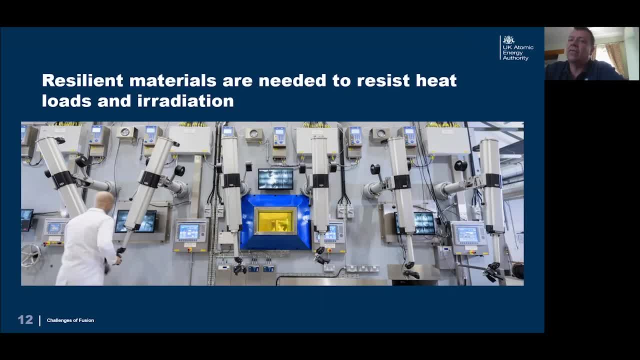 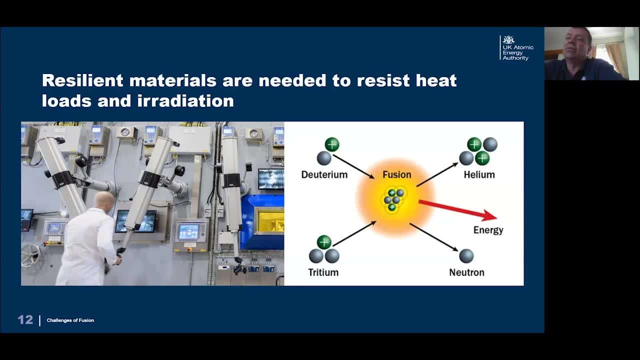 and will be absolutely key- working with universities as well to find and develop cleverer materials for our uses. So what are the particular challenges here? Here is a reminder of the fusion reaction: Deuterium and tritium sticking together to form helium and a neutron. 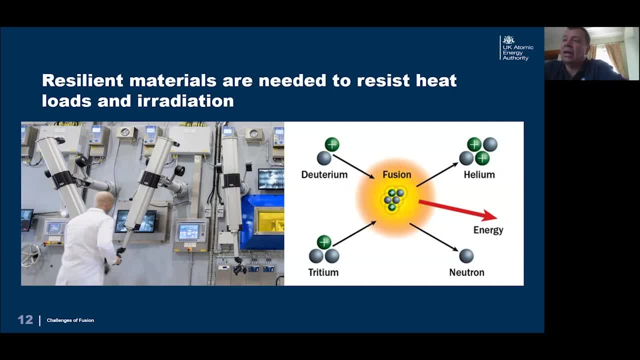 The helium stays in, as we just discussed, and we need to exhaust it out. when it gets cold. through the diverter, The neutron flies out. That is what captures most of the fusion energy: 80% That will fly out. It has no charge. 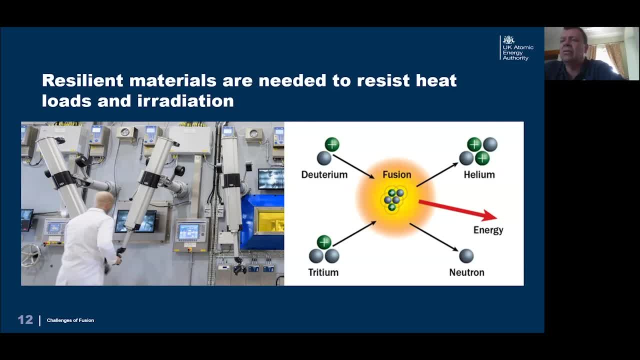 It doesn't care. There's a magnetic field there and it will penetrate into the material structural surfaces of the fusion power station. The steels or whatever we use to make the structure of the power station is not something that we can get out of. 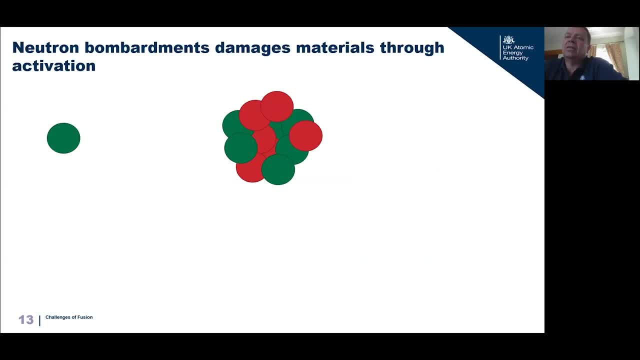 There are several issues there. Here is a neutron and here is a standard metal atom. It would have actually more protons and neutrons than that, but a heavier atom of some kind of structural material- The first thing a neutron might do. 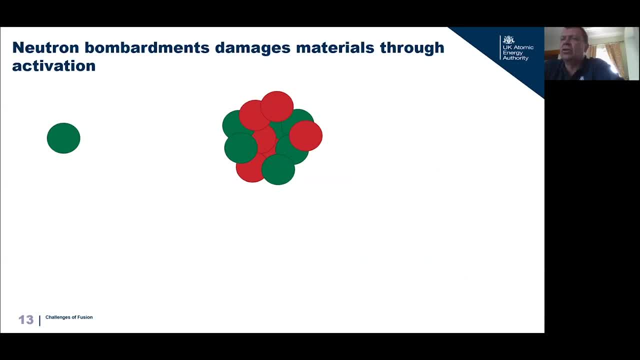 most of them will just pass past these atoms and start to slow down through collisions and give up their heat to the surfaces. We'll come on to how that works in the next talk. But it can cause damage and it can cause irradiation. 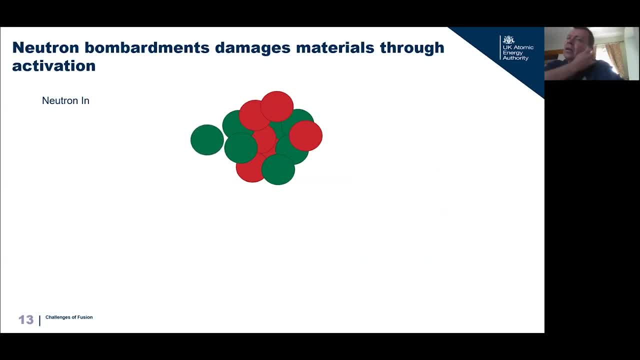 What a neutron might do is this: It might get absorbed into a particular metal atom And in some cases that will give radiation out. Let me just give you an example of that. If we use Inconel, which is often what we use, 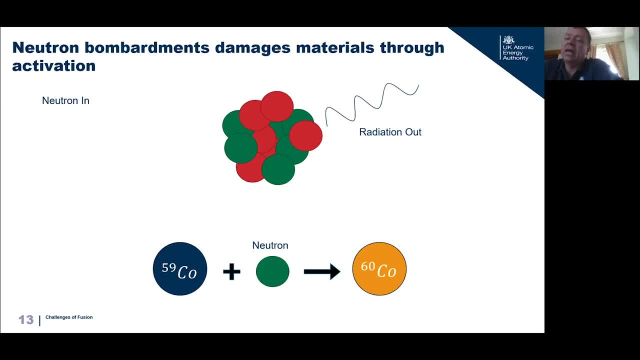 certainly for Marston jets or other types of steel. they contain some elements, some amounts of cobalt. Most of these materials do. Cobalt has 59 protons and neutrons and is utterly benign. But if it captures and picks up a neutron, 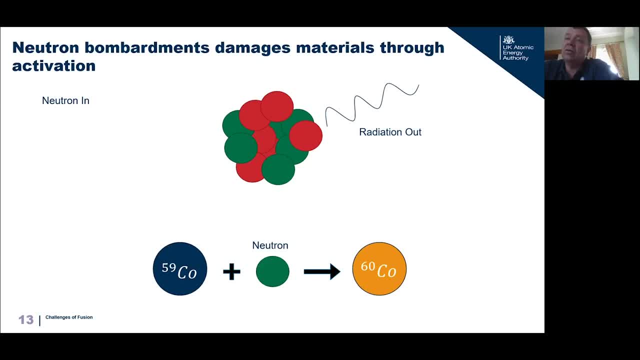 it turns into cobalt-60.. It's gained an extra nucleon, It's gained a neutron, It's now an isotope of cobalt, And cobalt-60 is a radiation emitter, Whatever we make our power station out of. 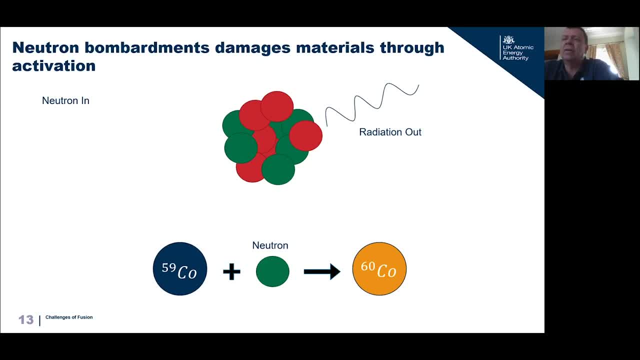 it is unlikely we'll find any material mix that will be immune to this picking up of neutrons and this radiation production. But it is in our gift, if we're clever and we can find the right materials, to find materials that don't get too active. 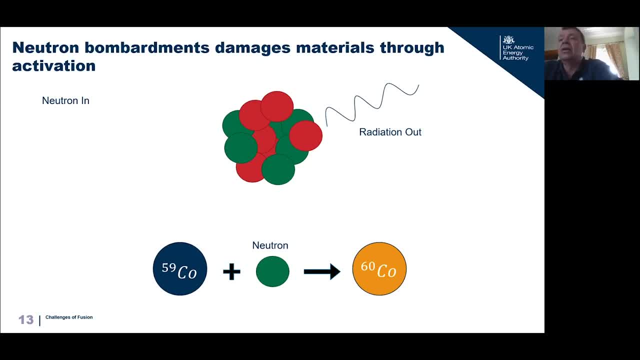 or that if they do, the activation dies off quite quickly. This is less long-lived than activation from fission, but we wish to find materials that would minimize the activation. right now Impossible really to consider no irradiation, but certainly minimize that radiation. 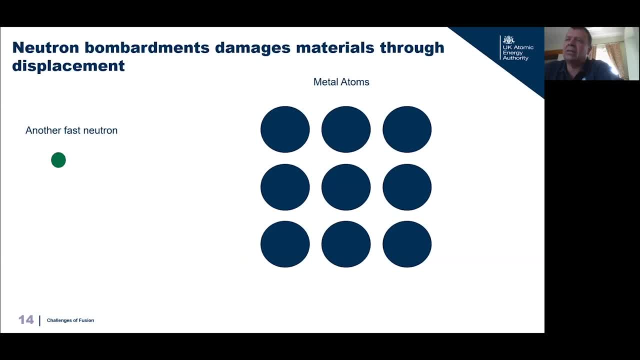 The second issue, and here is a group of metal atoms, each, of course, containing all those protons and neutrons. we just spoke about The other thing a neutron might do, because they're very, very fast, 10 times faster than the neutrons. 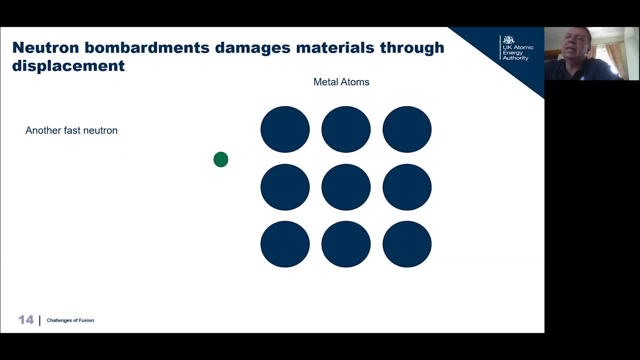 from standard nuclear fission is that it can easily do this. It won't do it all the time, but we know that a neutron can knock an atom out of place. Metal atoms are very carefully arranged in a very structured and uniform structure. 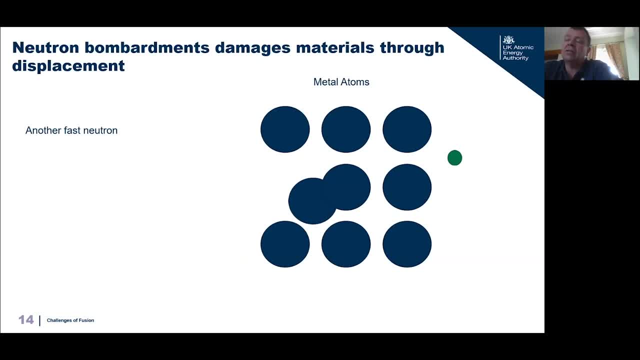 just like this, where they're all lodged on top of each other and next to each other, very closely bound. That's what makes a metal very strong. By the action of the neutrons, we'll start to knock atoms out of the way. what we call displacements, and we'll end up with a weakened metal structure Again. if we can find materials that are particularly resistant to these particular neutrons, that will help us hugely in devising structural materials that will last for the 40 or 50 years we need them to. 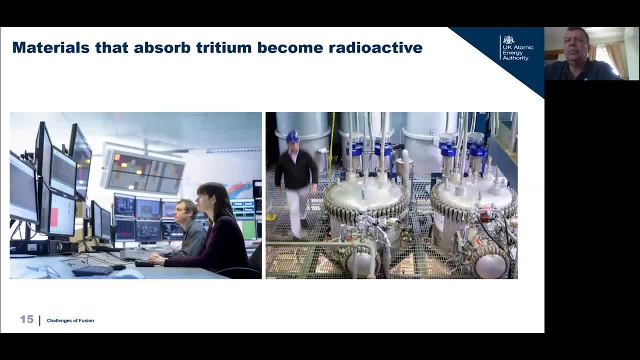 in the environment of these very fast neutrons. Finally, the very first wall materials, those tiles that we saw on Jet particularly, are prone to absorbing fuel from the plasma. We have deuterium and we have tritium. We don't really mind too much if it absorbs deuterium. 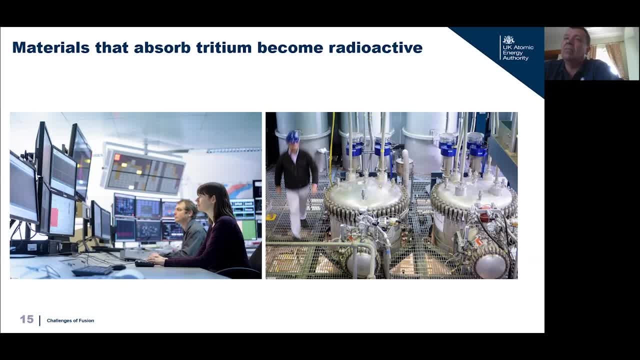 that's neither here nor there. If they absorb tritium too much, they become really quite active in their own right. Tritium is a radioactive gas. it's a radioactive isotope of hydrogen. has a decay time of about 10 years. 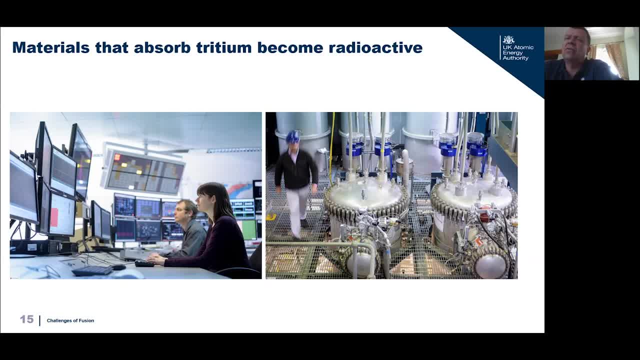 half disappears in 10 years. but we just don't want tritium fuel in the tiles in the plant itself. we want it fusing in the plasma Machines like Jet. indeed, when we were looking decades ago to power plants, 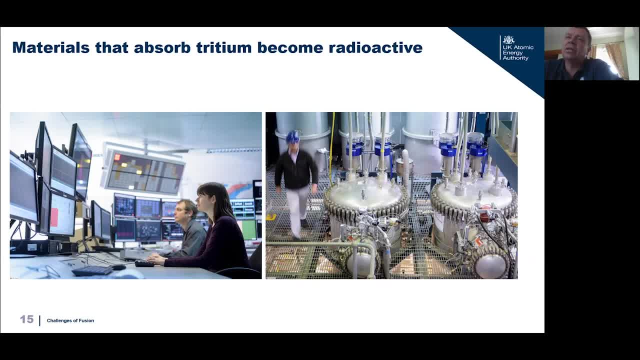 we wanted to use carbon. Carbon was a very good first wall material for many reasons, but its Achilles heel was its ability to suck in tritium and hold it, and we didn't want that to be the case. This is why we chose 10 years ago now. 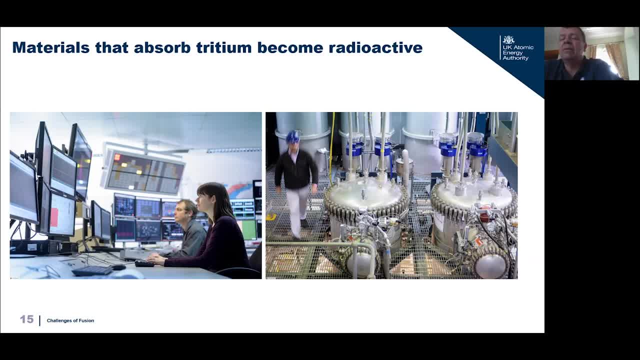 to change the whole wall structure on Jet to beryllium, which is much more immune to absorbing that tritium and tungsten at the very bottom in the diverter. So we're actively looking for materials that resist absorption of tritium. 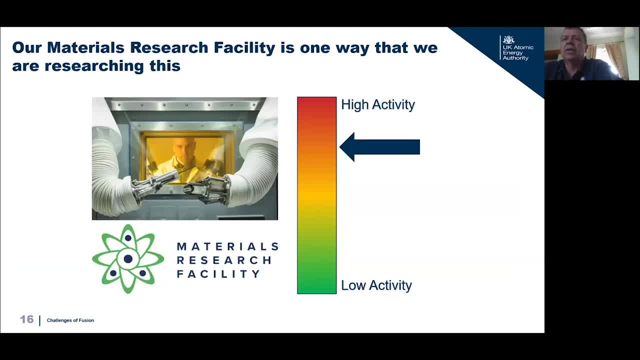 because we don't want to activate the machine too much And our materials research facility is looking into these materials issues, in particular the radiation and damage. We can take structural samples that have been irradiated by fusion energy neutrons in other facilities. 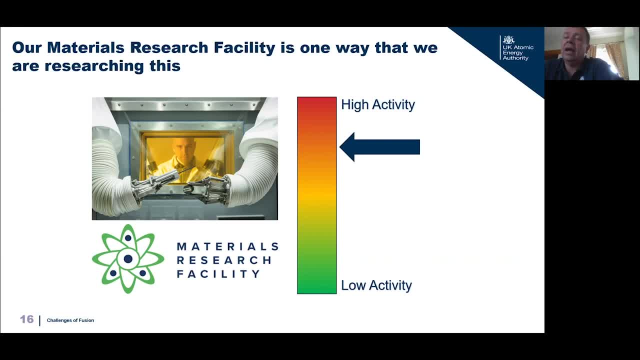 The MRF gives us the ability, on a very small scale, to test how weakened they have become. How can we do that? We can take really very active samples, but we're not a licensed site, of course, at Cullum. Neither would we wish to be ever. 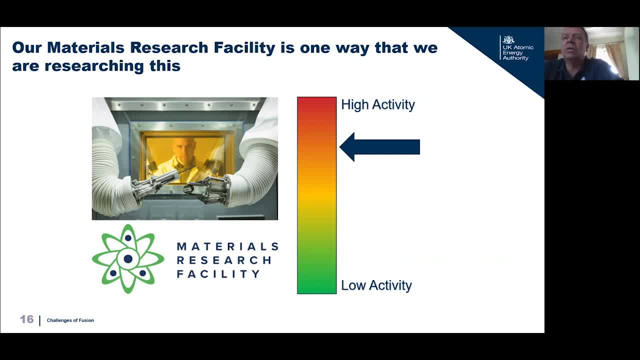 We can do that because we only can take in very small material size samples of these very active materials. So we are in the middle towards the high active range of materials. Low activity, structural work and materials testing can go on in universities. We sort of stand in the middle ground. 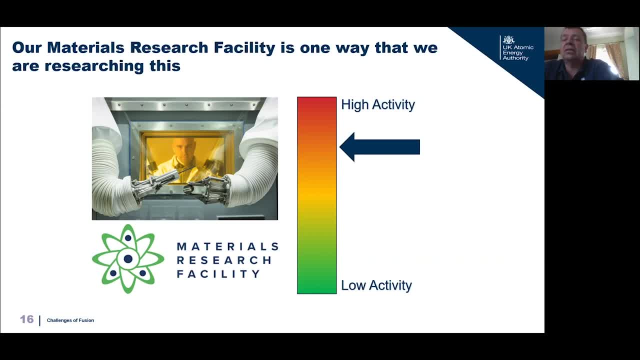 The very high active end is where Sellafield can test very big components. So there's an overlap here with the MRF, with the fission industry. but they can look at candidate fusion materials And we really hope the MRF will play a role. 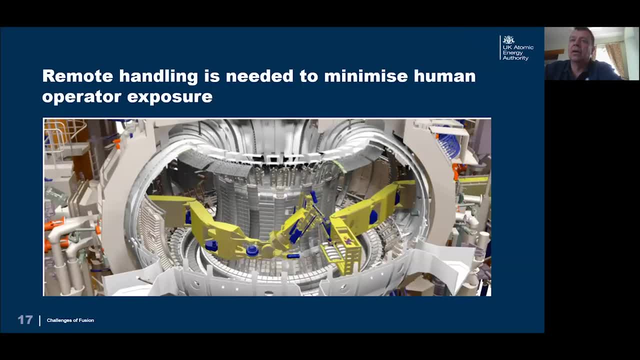 in developing these materials in the future. Finally, we're just going to talk very quickly about remote handling. We have a remote handling system in JET. JET is unique in the world in Tokamaks of having a remote handling system. 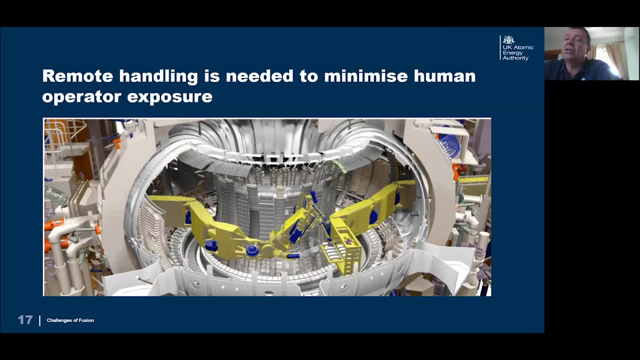 And we've been able to demonstrate doing pretty much anything in vessel changing tiles, aligning things, lifting in new equipment, even hoovering up after themselves. The boom inside JET does absolutely amazing things. On the left you can see the boom coming in. 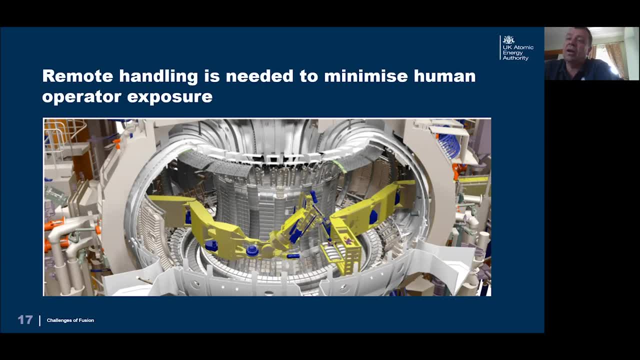 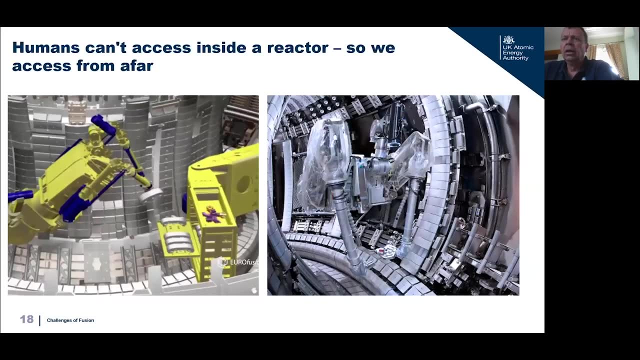 and it works very often in tandem with a second boom bringing in fresh equipment, taking out old stuff to be stored and monitored. But in future fusion power stations we'll need even cleverer robotics to look on the outside of the machine as well as the inside. 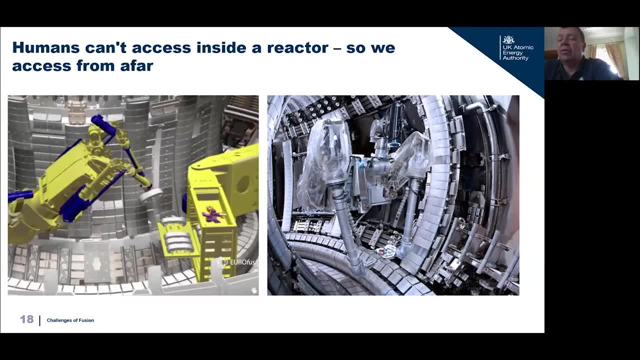 Here is a better picture of the boom inside JET On the right hand side you can see it very much mimics a pair of arms. If you've never seen this, when we certainly get back to site, we'll try and do a show and tell. 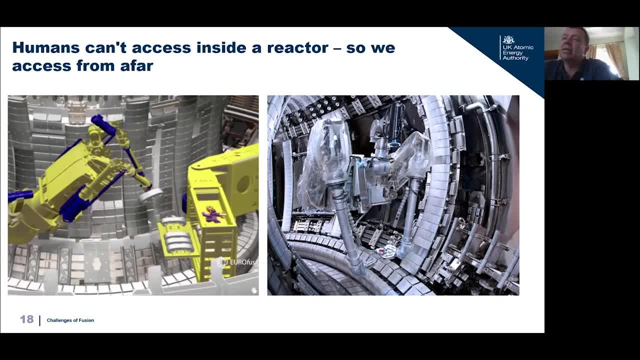 where we can show off the remote handling gear in action. It is quite amazing. There were operators 50 meters away operating the main end of the boom and the real boom inside the machine will do exactly as they're telling it to do, So they can do very complex tasks. 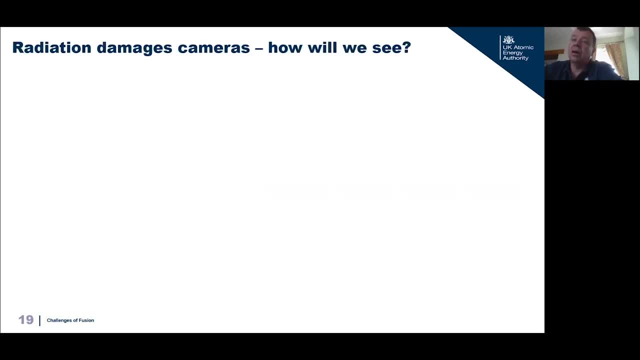 for this remote handling system But we do not use that On the outside of the machine. remote handling systems on ITER will have to test how we can fix things on the outside of the machine as well as the inside, because in ITER and future fusion power stations 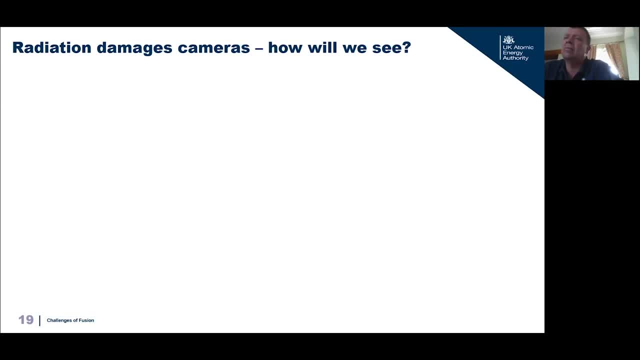 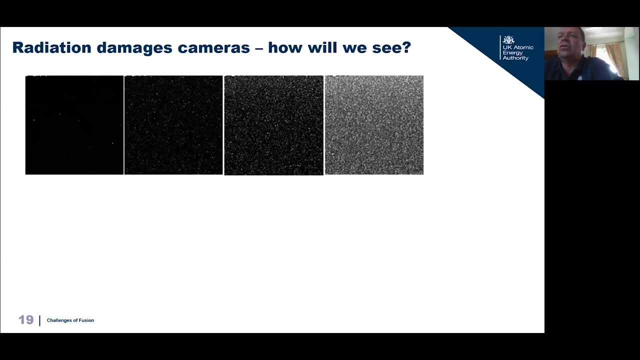 the activation levels will be higher. We're gonna need to work remotely much wider range. The other issue is that the radiation, certainly the radiation caused by neutrons, can damage standard cameras. If we're gonna rely on a standard set of cameras to look inside and control the remote handling. 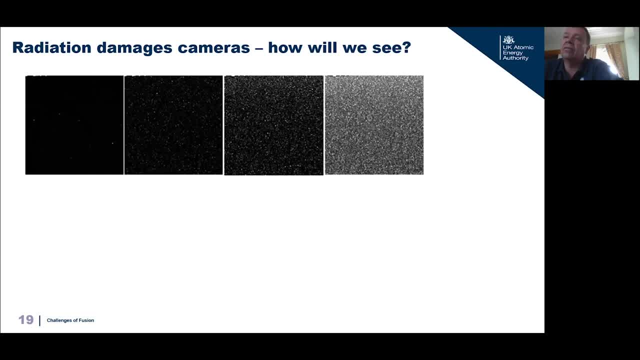 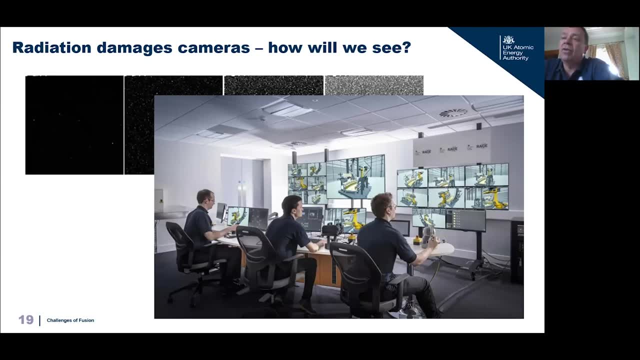 this is what happens, What happens to cameras when they're subject to intense fusion radiation: they start to white out. So we are developing, and RACE is developing, really clever virtual reality systems. They already use virtual reality a lot in operating in JET. 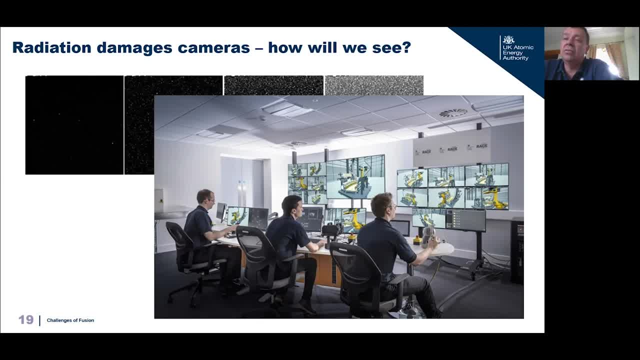 but trying to devise control systems that can link a robot with the users in as absolutely a seamless way as possible, cutting out any kind of analog signals and camera views and using virtual reality in almost all regards. So some really clever stuff up at RACE. 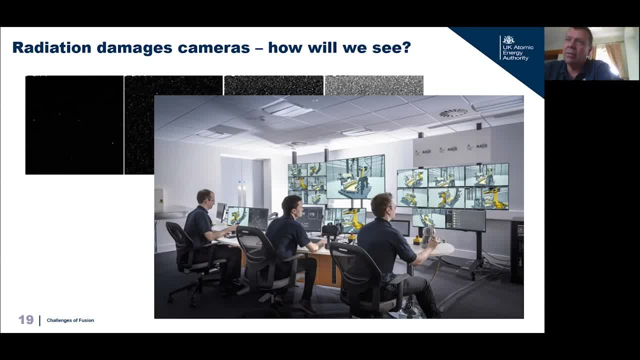 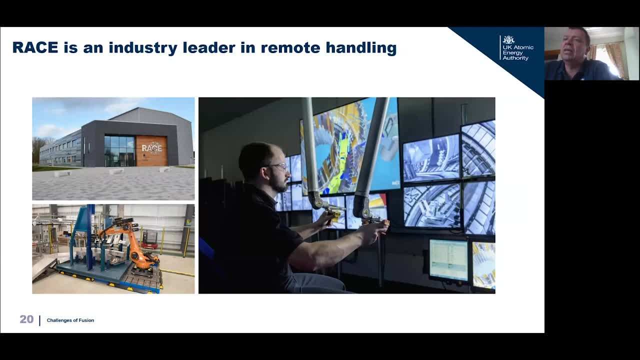 Looking at what future systems might look like, helping with industry to design systems for ITER and looking beyond to the first power stations. And it is really a genuinely industry leader. It's grown hugely over the last three years, RACE Starting now, if you can look in the bottom left. 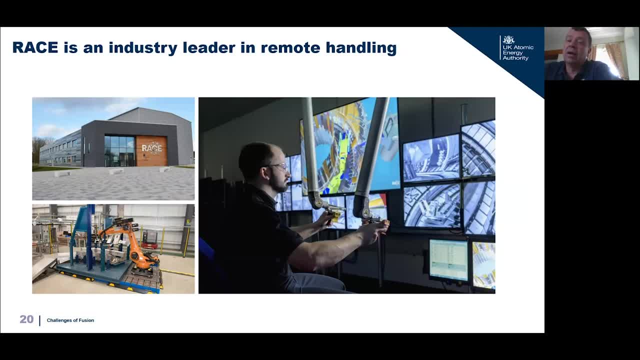 to link up industrial type robots. this is a KUKA that will be on the line at the car factory with a fusion environment, so that we can bring this much more mainstream. devise these clever control systems, but devise robotic systems that can be used in the future. 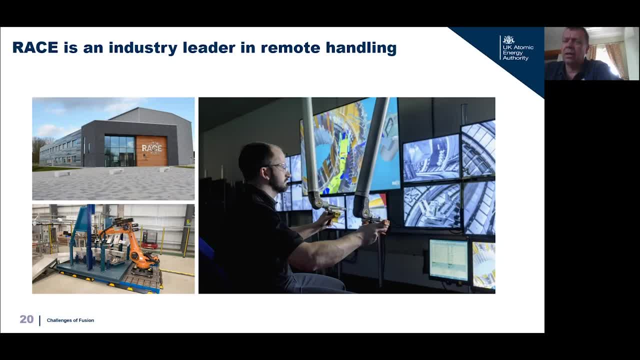 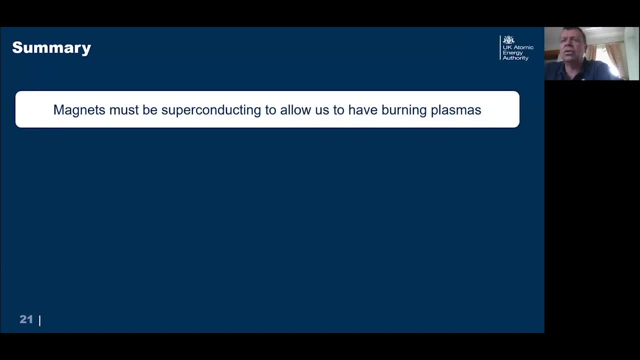 So that's what we're trying to do. We're trying to build systems with industry that can work in ITER and future fusion power stations. So finally, a very quick whistle stop through Some of the major technology issues that we have to face.